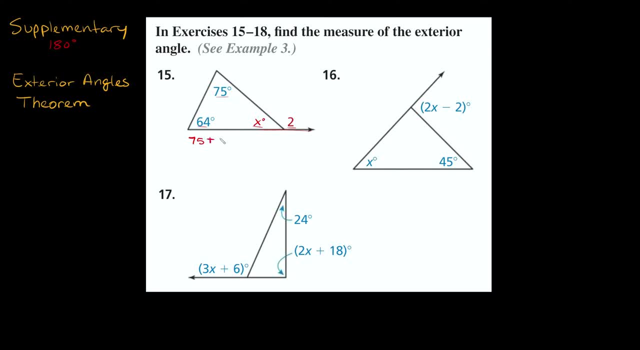 right. So 75 plus 64 plus x degrees should equal 180, right? So then, to solve for x right here, we can just subtract 75 and 64 from this side right And move it onto this side, So we're going to have x is equal to. 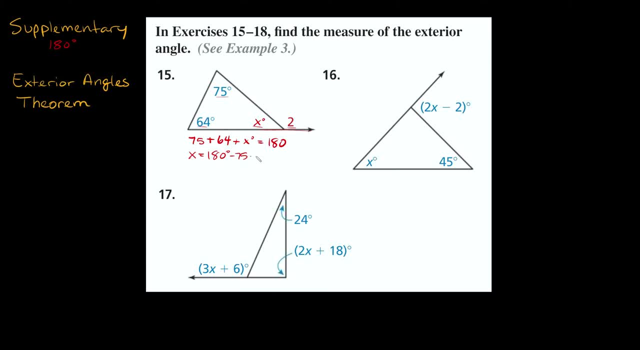 180 degrees minus 75, minus 64,, okay. So then here x is going to be equal to 41 degrees, okay. So we just figured out what this angle is. right, It's 41 degrees, 41, degrees, okay. So again, this angle right here, the 41 degrees, and this exterior angle out. here are 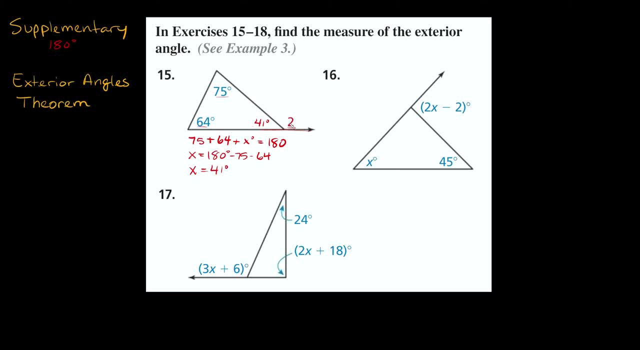 supplementary. So if I add them up together, they should add up to 180 degrees. So then 41 plus this missing angle, which is labeled as 2, that's kind of confusing, though. right, Let's just label this as y, right? So then y. so 41 plus y is equal to 180 degrees. So then to solve for y, right here. 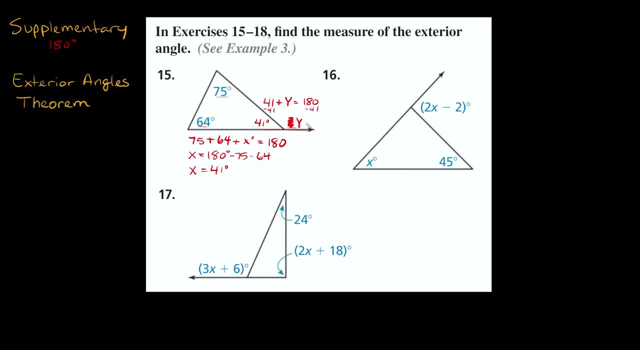 subtract 41 from both sides subtract 41. So then we get: y is equal to 180 minus 41, which is equal to 139,. okay, So then this angle right here is equal to 139 degrees. All right, so that was the first method that you 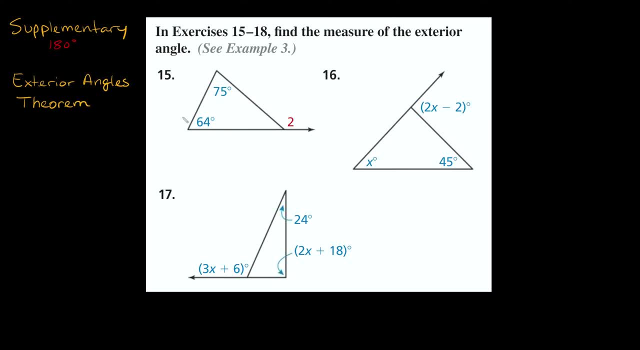 can use Now. the second method is using this theorem right here, the exterior angles theorem, And it just says: whenever you add up the interior angles over here, they add up to this exterior angle over here. all right, As long as you add up the interior angles over here, they add up to this. 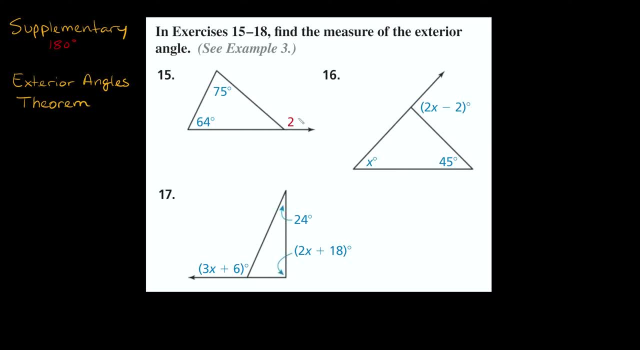 exterior angle over here. So that means that the angle that it gives you is not next to the one that you're trying to find out here. So, as you can see, the two angles over here that it gives us are not next to, it's not touching, it's not supplementary to this angle right here. that 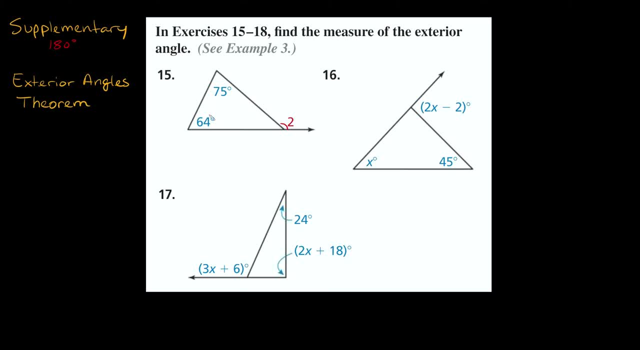 we're trying to find right, So that means we can use this theorem, okay. So again, all you have to do is add up these two, and it should add up to the angle that's out here. So 75 plus 64 is equal to. 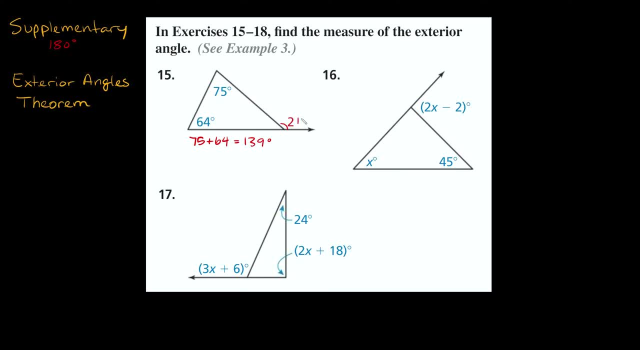 139 degrees. okay. So then that means this angle out here is 139 degrees. okay. So we got the exact same answer as we did with the very first method, right? But again, this method only works if the two angles that you're given are not touching. 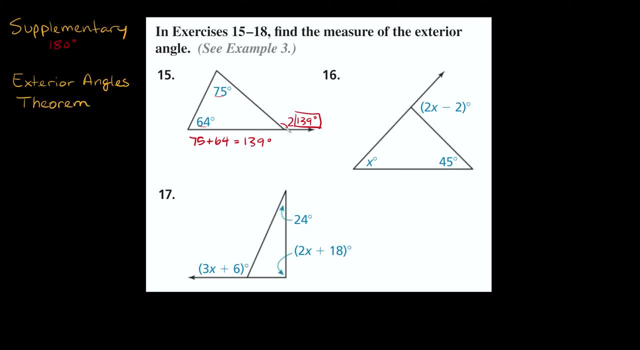 they're not next to, they're not supplementary with this angle, this exterior angle that we're trying to find, okay. So, for example, let's say this 64 degrees wasn't here. Let's say this wasn't given right, Let's get rid of that there And let's say instead that the 64 degrees was. 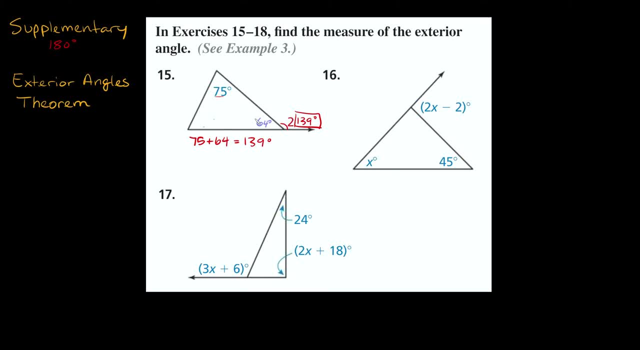 right here. Okay, so if the problem was set up like this, then we can't use this exterior angles theorem, because the angle that it's giving us, that it's given, is next to the angle that we're trying to find. okay, So if the problem was set up like this, you would definitely have to use the first method. 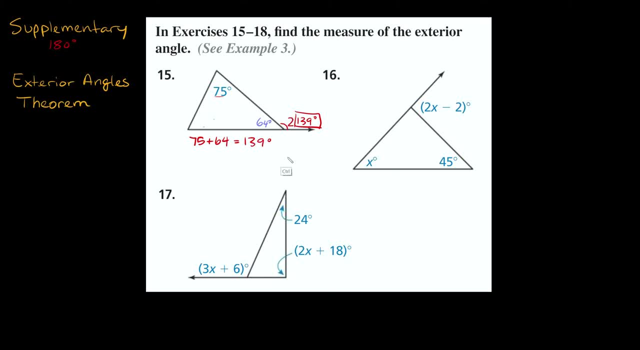 just trying to use supplementary angles, right, But that wasn't the case in this problem, right? So that's why we can use the exterior angles theorem And for the other few examples that I'm going to go over, we're going to use the exterior angles theorem for all of them. 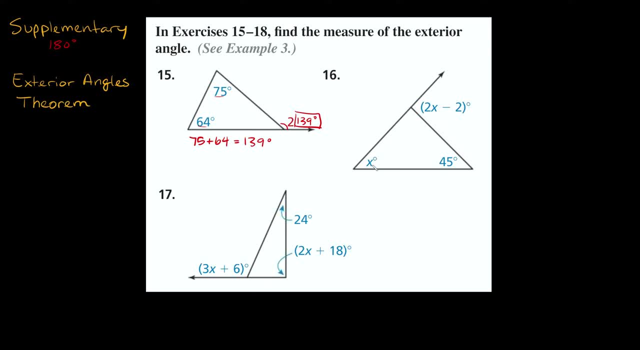 Okay, so it's pretty straightforward, right? So let's go to this next example: right here, So 16, right? So we have two angles right here, so x degrees and 45 degrees, and then this angle out here, 2x minus 2.. So, as you can see, the two angles that it gives us right here are not next to this. 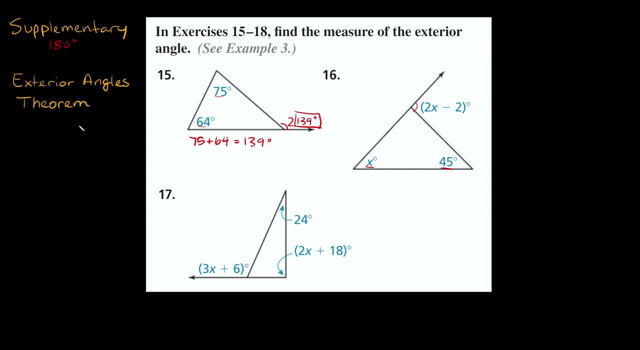 exterior angle. right here, right. So again we can use the exterior angles theorem. okay, So again, that just says that the two angles on the inside, when you add them up, should equal this angle on the outside. Okay, so if we do x plus 45 degrees, that should equal this one out here, 2x minus 2.. 2x minus 2.. 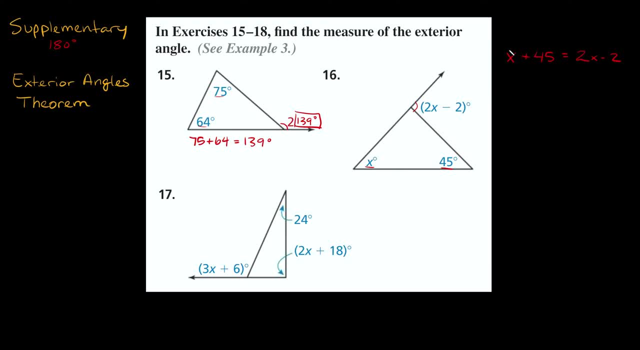 Okay, so we're trying to isolate the x's on one side of the equation, So let's move this x over here, right? So we're going to do that by subtracting. So subtract x from here, and what we do to one side, we do to the other, right? So we'll subtract x from here also. And then these: 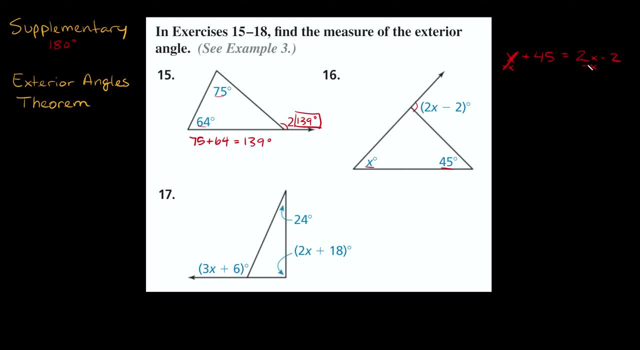 x's cancel out. So then over here we have 2x minus x, which is equal to 1x, right? So that's equal to 1x minus 2.. So then we're left with 45, right Positive 45 is equal to 1x, or we could just: 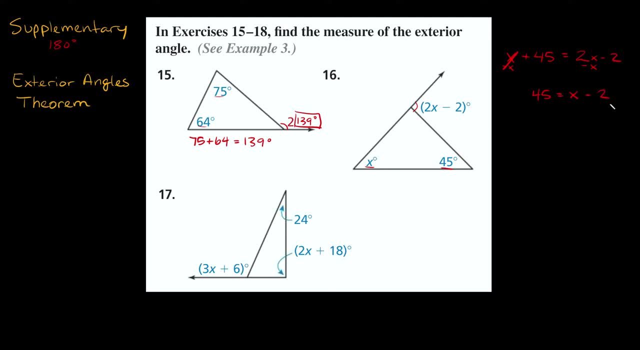 write that as x minus 2.. Okay, and then we'll get rid of this minus 2 by moving it to the other side. So add 2 to both sides, right? So then these cancel out. So then we're left with x is equal to. 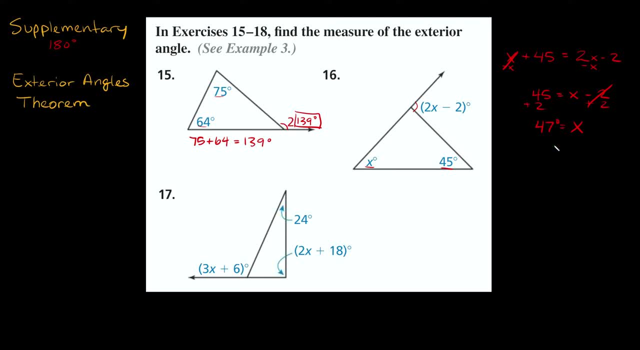 45 plus 2, which is equal to 47.. All right, so now that we know what x is equal to, the easy way to solve this would just be plugging it straight into the exterior angle: the 2x minus 2 over here. But. 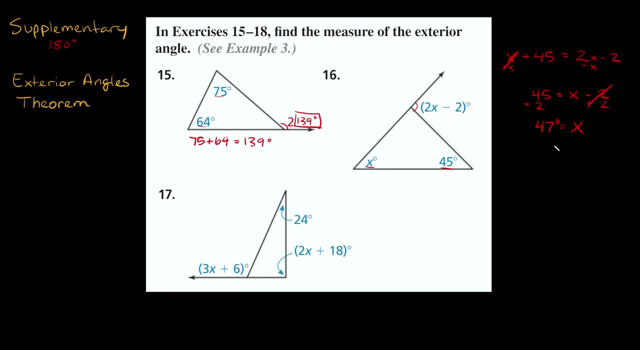 I'm actually going to plug it into the exterior angle. So I'm going to plug it into the exterior angles and then add them up, just so I can show you that you'll still get the same answer either way. all right, So x is equal to 47 degrees. all right, So that means this angle, right here. 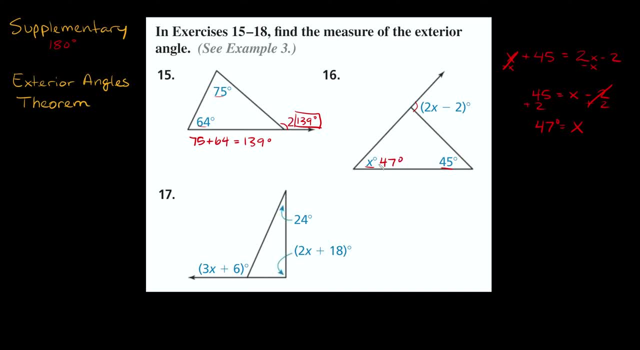 is 47 degrees. Okay, so now that we know our two interior angles, right here again, we can just add those up: 47 plus 45, and it should equal this angle out here. So 47 plus 45 is equal to 92, right, So then this angle out here is equal to 92 degrees. 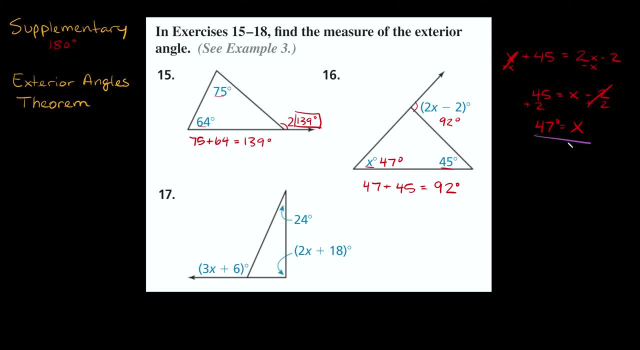 Okay, and if we want to check our answer right here, right x is equal to 47 degrees. we can just plug this into this little equation right here. And again, it should be equal to 92 degrees, right? So let's write it over here: So 2x minus 2 should be equal to 92, right? So let's? 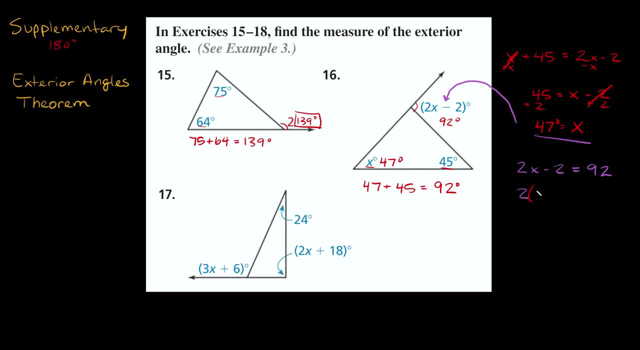 plug in what we got for x. So we got: 2 times 47 minus 2 is equal to 92, right? So 2 times 47, that's equal to 94.. Okay, so then we get 94 minus 2 is equal to 92.. So then we get 92 is equal to. 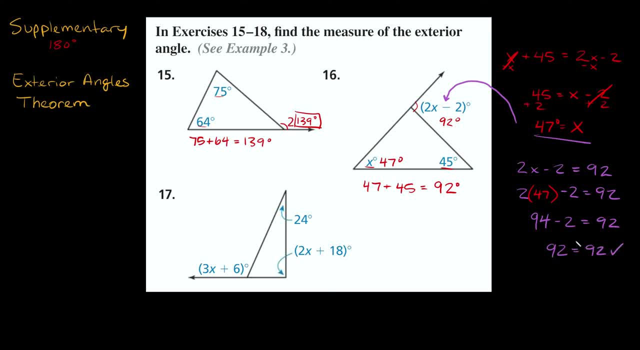 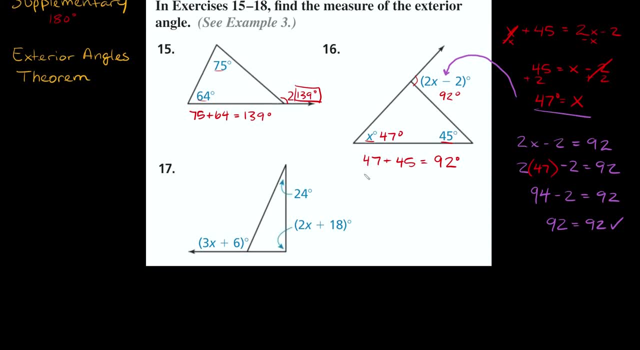 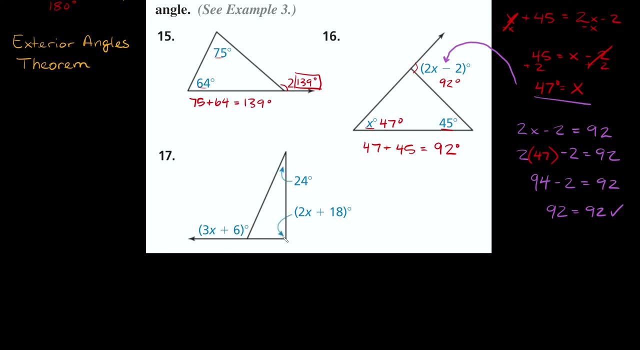 92, right. So we got the correct answer for our x, because our equation balances out right, Checks out. Okay, and I'm going to scroll down a little bit for this next one. So number 17,. all right, So again we have our two interior angles right here, right: 24 and 2x plus 18.. So 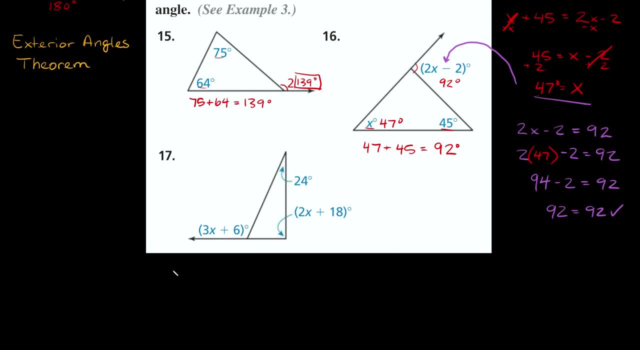 when we add these up, they should equal this exterior angle right here. So we're going to do 24 plus 2x plus 18.. And that should be equal to our exterior angle 3x plus 6.. So the first thing. 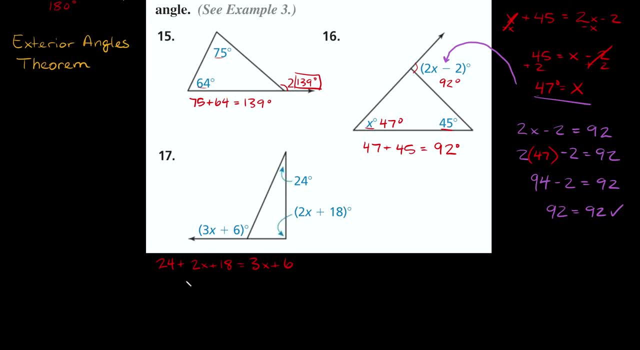 you always want to do is try and get your x's on the same side. So we have a 2x over here, positive 2x, right. So we'll subtract 2x from this side And what we do to one side of the equation. 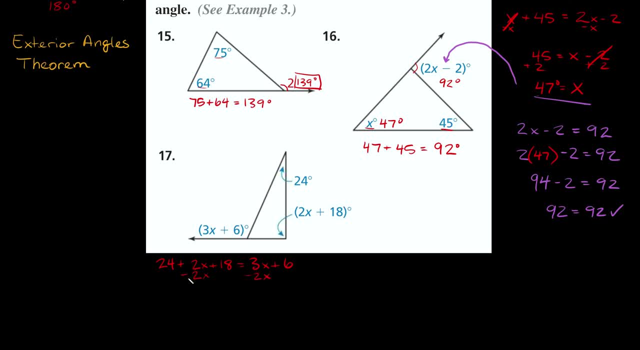 we do to the other. Okay, so then these cancel out. And then on the left side over here, 24 plus 18. And that's equal to 42. Okay, so we got 42. And then that's equal to right, equal to. 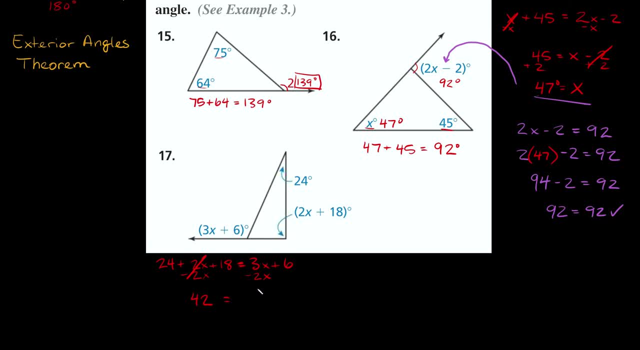 3x minus 2x, which again is just equal to 1x, which we can write as just x, like that, and then plus 6.. All right, so then to solve for x, right here, we'll subtract 6 from both sides. Okay. 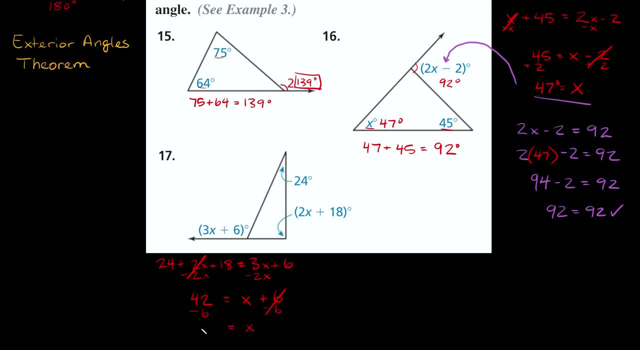 these cancel out. So then we get x is equal to 42 minus 6,, which is equal to 36.. All right, cool. So we got x is equal to 36.. So again now that we know what x is equal to. 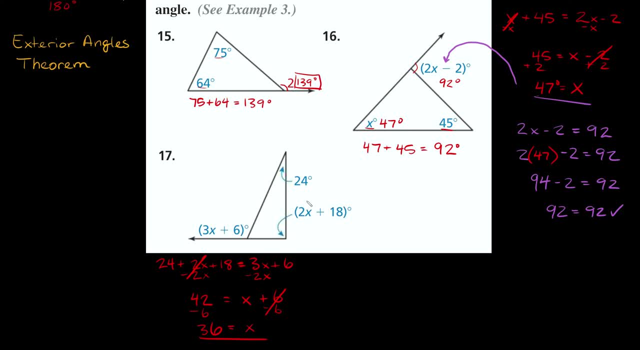 the easy way would just be plugging it in straight into the exterior angle, the 3x plus 6.. But I'm going to plug it into these interior angles one more time, just so I can prove to you one last time that adding these up will get you the same answer. So then we'll plug in a 36. 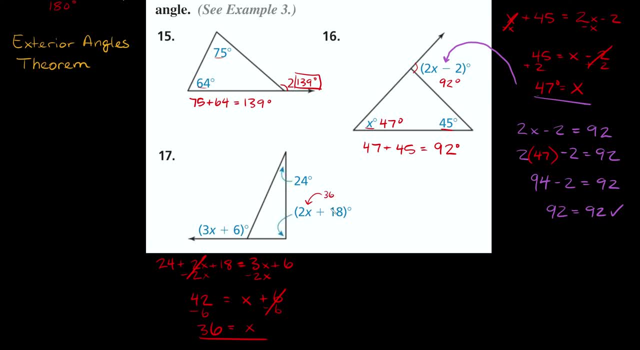 for x right there. So then we can figure out what this angle is over here. Okay, so then we'll have 2 times 36 plus 18.. So 2 times 36, that's equal to 72. So we got 72 plus 18,, which is equal to. 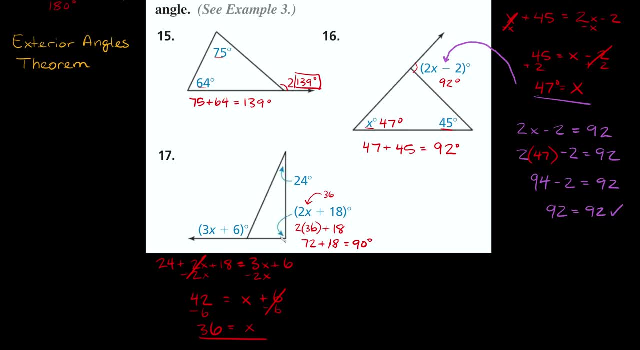 90.. Okay, so then this angle right here is a right angle. actually This is a 90 degree angle, right? So we got 90 degrees right here, 24 degrees up here. So again we just have to add: 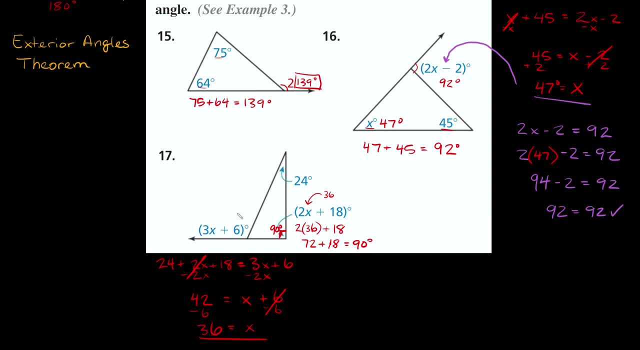 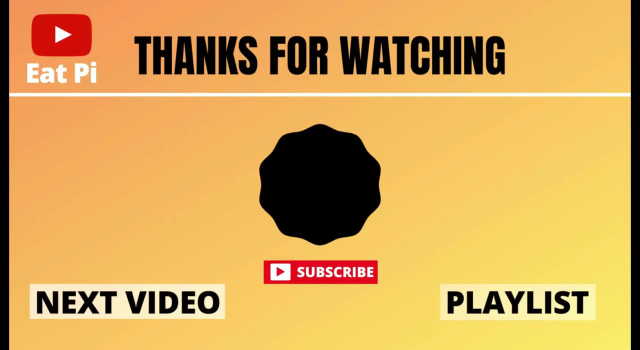 these two up to figure out what our exterior angle is out here. right, So we can do 24 plus 90, and that's equal to 114.. Okay, so then this angle right here is equal to 114 degrees. So if you found the video helpful, definitely leave a thumbs up down below, And if 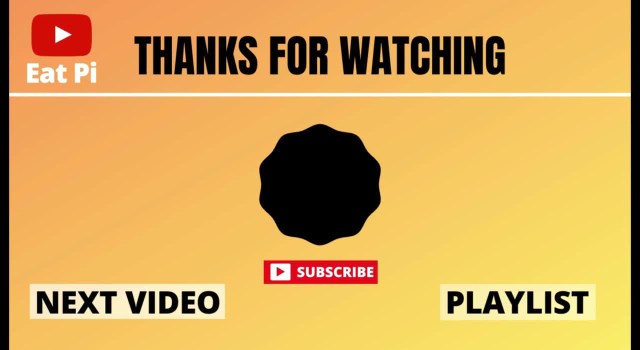 you have any other questions or want to see any other examples, just let me know in the comment section below.